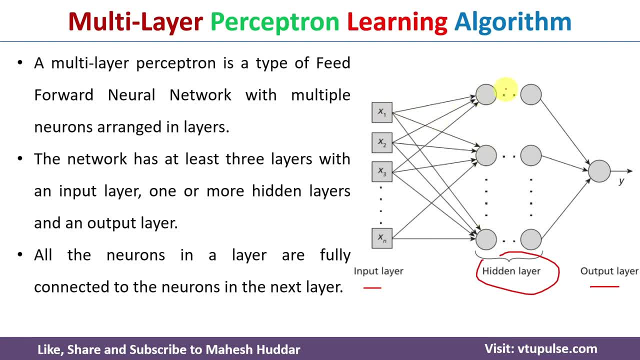 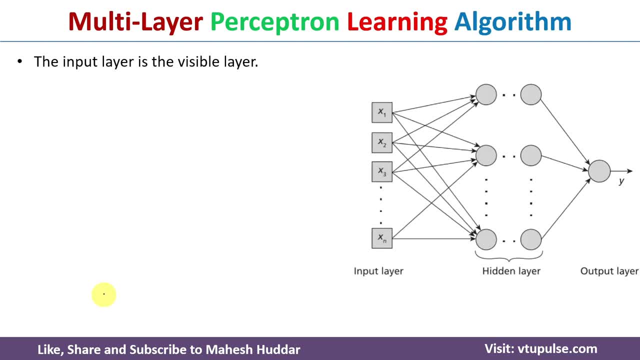 the next layer. Similarly, if we consider this neuron, it is connected with each and every neuron in the next layer, and so on. So that is what is called as fully connected. in this case, The input layer is the visible layer, ie the input is given at this particular layer. It. 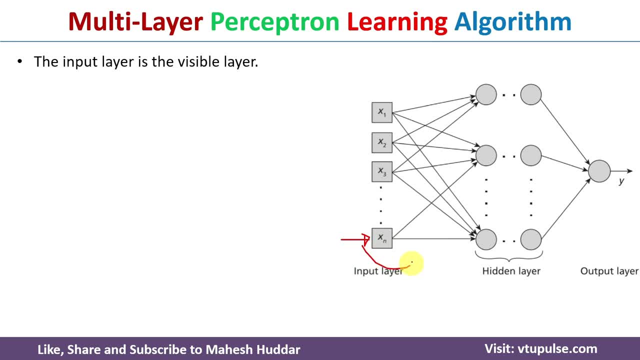 doesn't do any task over here. Whatever the input is received, that will be transformed to the next layer. That's it. It will not do any modification to the inputs, It will just transform that particular input to the next layer, And then the hidden layers will not receive input directly or they will not give the output. 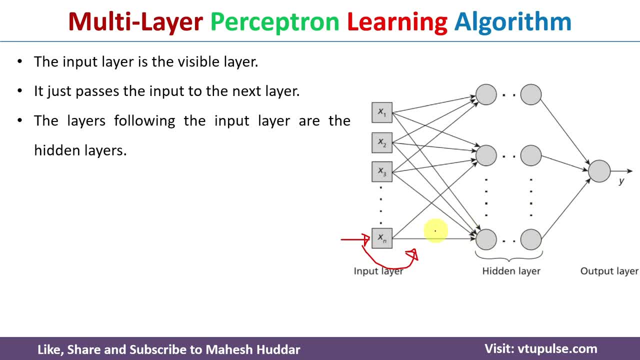 to the environment here. They will receive the input from the previous layer and then they will do some modification. That output will be given to the next layer, and so on. Now the output layer will do the computation after receiving the input from the last hidden. 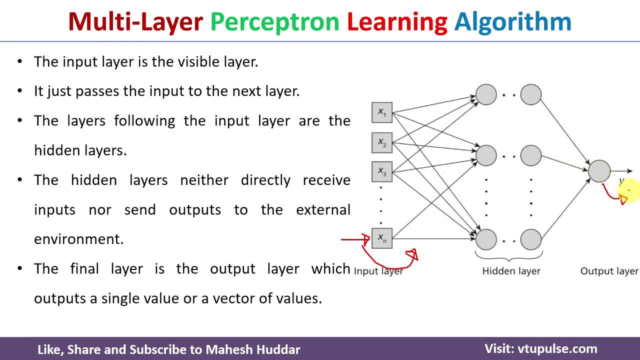 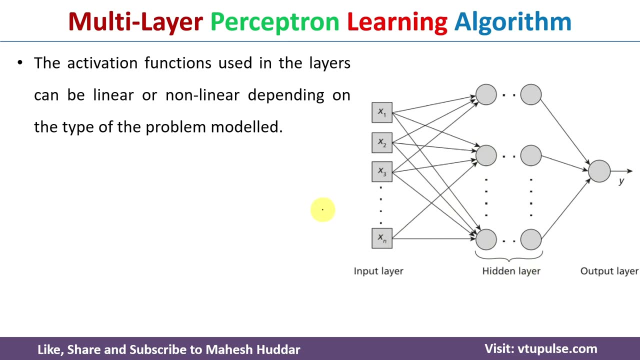 layer and then it will output that to the environment in this case. So the input is given to the network through the input layer and the output is received from the output layer neuron. in this case, For each and every neuron in the hidden layer, we need to use the activation function. 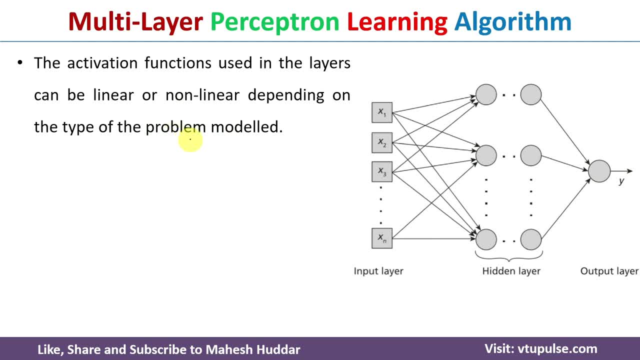 There will be multiple kind of activations. Activation functions exist: linear, non-linear, and so on. Based on the problem definition, we need to use different activation functions. I have already discussed the different activation functions in artificial neural network. The link for that video is given in the description below. 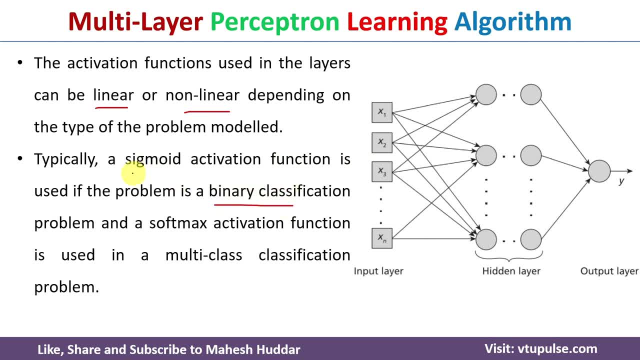 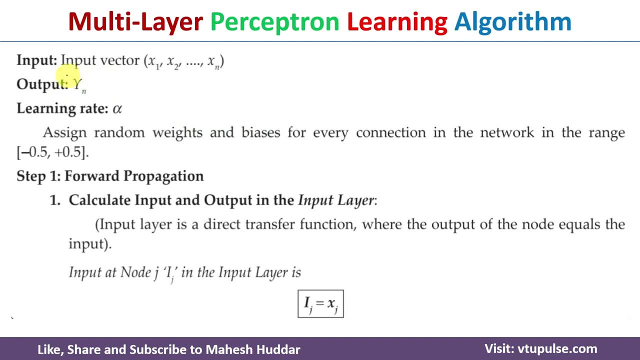 Usually, whenever we have binary classification problem, we use sigmoid activation function. If it is a multiclass classification problem, we use softmax activation function. Now we will discuss. The input to the multi-layer perceptron learning algorithm is input vector. that is the set. 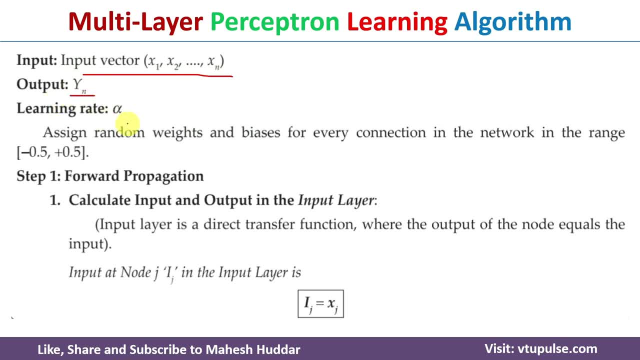 of features and output is the target in this case. We need to define the learning rate alpha here and for each of those we can say that the edges- we need to assign the weights as well as the biases. over here. Usually we will assign the weights and biases randomly in the range of minus 0.5 to plus. 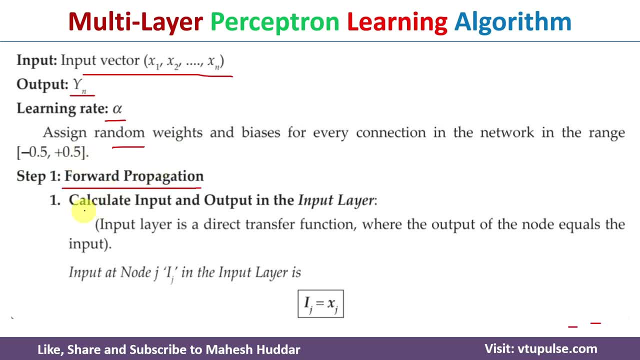 0.5. here In the first step of forward propagation we need to calculate the input and the output at the input layer. So input calculation is whatever the input is given to the network, that is the input and output of that input layer. neuron is nothing but the direct transfer function here. 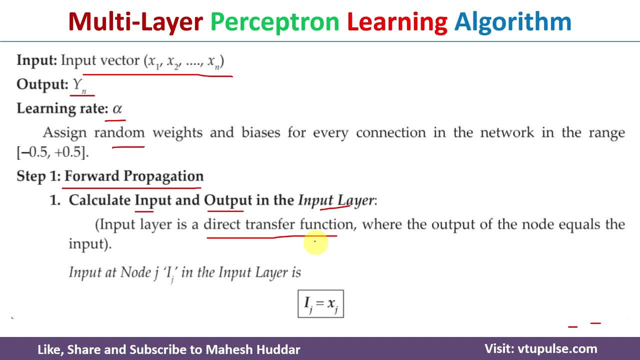 That is nothing. but whatever the input is there, the same thing will be transferred to the next layer in this case. That's the reason: the output of this input layer is exactly equivalent to the input to that particular input layer- neuron in this case. 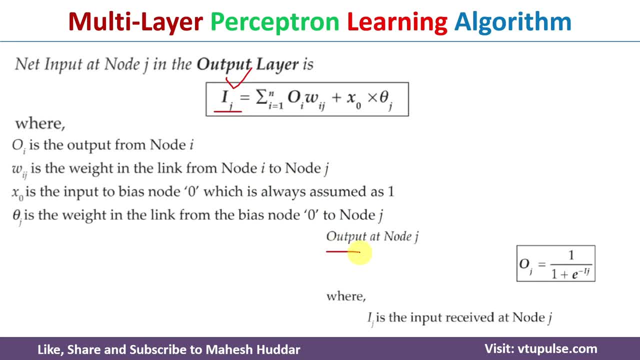 calculate the net input. the next step is to calculate the output at that neuron. again, it is based on the activation function. we are using, in this case the activation function. what i have shown here is nothing but the sigma activation function here, oj, that is, output is always equal. 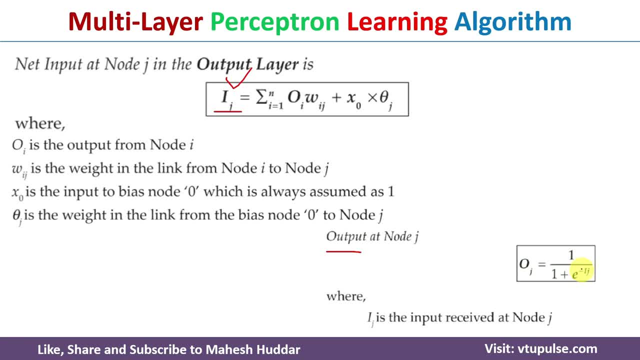 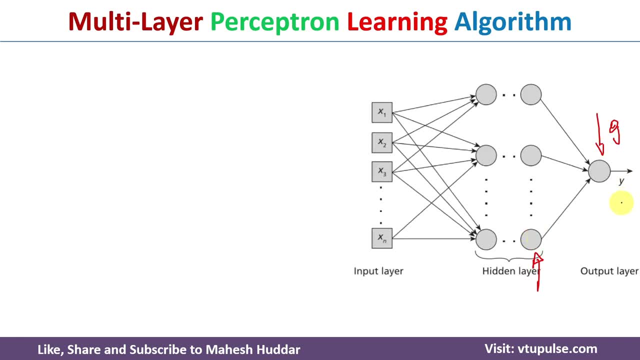 to 1 divided by 1 plus e raised to minus the net input. here net input is what ij. so if you put that particular thing you will get the output at the output layer neuron in this case. so we were able to calculate the output at the output layer neuron over here. now, once you calculate the 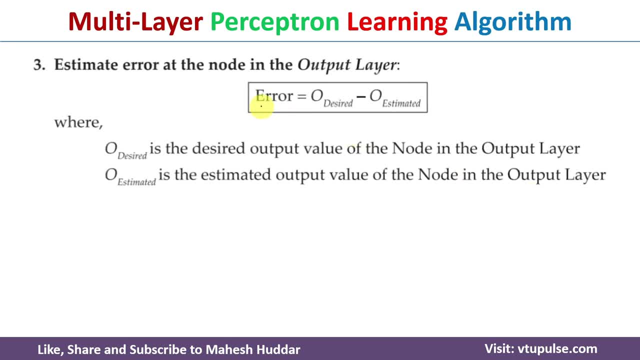 output at the output layer neuron. the next step is to calculate the error. so error is always equivalent to o desired, that is nothing but the target output, minus o estimated, that is nothing but the calculated output. so once you do this calculation, you are going to get the error term. 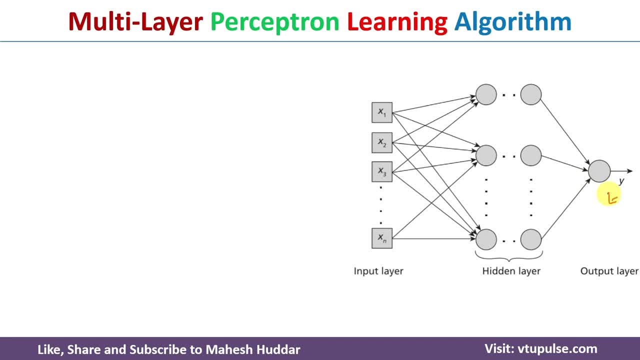 in this case. so once you calculate the error at the output layer neuron, what is the thing we need to do is we need to apply the back propagation algorithm, and then we need to apply the back propagation algorithm, and then we need to apply the back propagation algorithm, and then we need to propagate this error back side till the first hidden layer in. 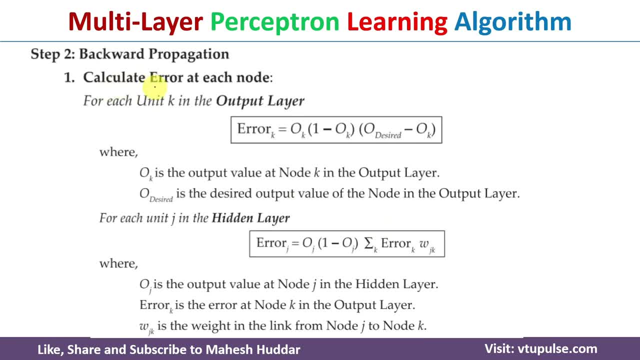 this case. to do that thing we use the two things over here. the first one is calculating the error at the output layer neuron, calculating the error at the hidden layer neuron here. these are the two different things we need to perform because, whatever the error, we have calculated that. 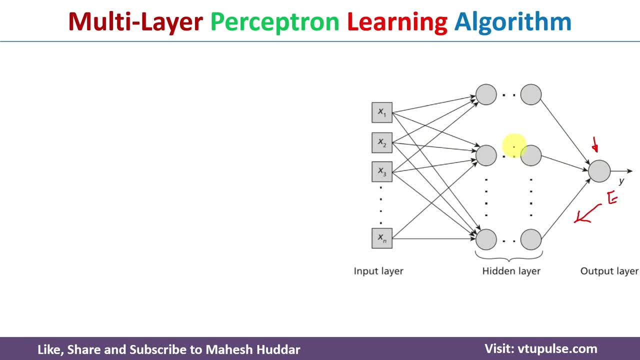 entire thing is for the output layer neuron. but when you look at this hidden layer neurons, whatever the error we have calculated here, that will be propagated back, propagated by the proportion of this particular weight. here, for example, weight is equivalent to 0.5, so 50 will be propagated back side. if it is equivalent to 100, it will be propagated at the. 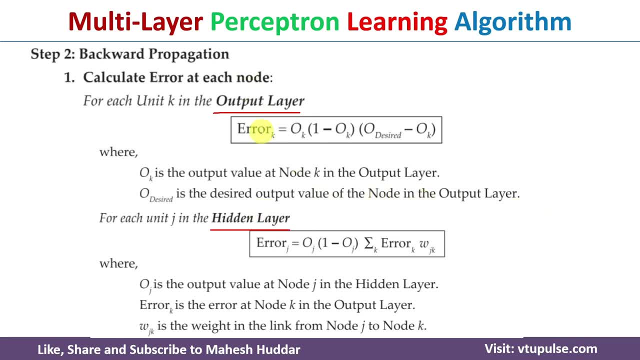 back side over here. so that is the reason we need to calculate these errors separately here. for error at the output layer neuron, this is the equation we use. error k: k is the output layer neuron here. okay, multiplied by one minus, okay, okay is nothing but output. we have already calculated. 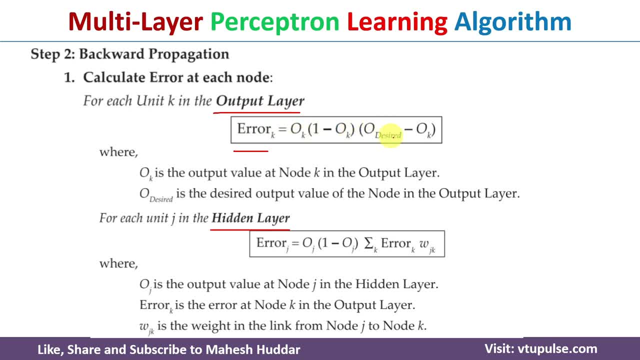 it one minus okay, multiplied by o dz, that is nothing but the target output minus okay again. we have calculated it. so once you calculate the error at the output layer neuron, what we do is we will calculate the error at the hidden layer neuron by propagating this error. that is the one. 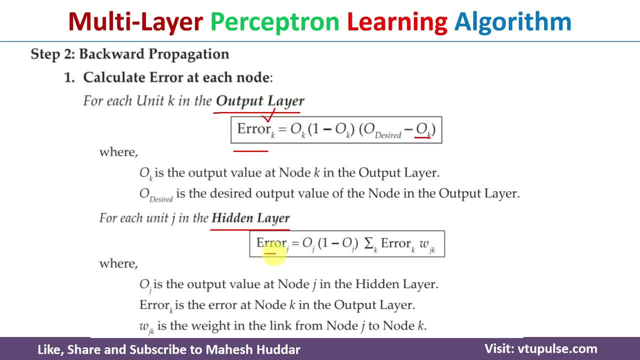 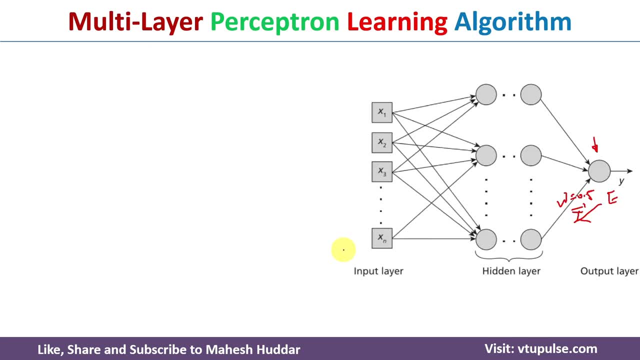 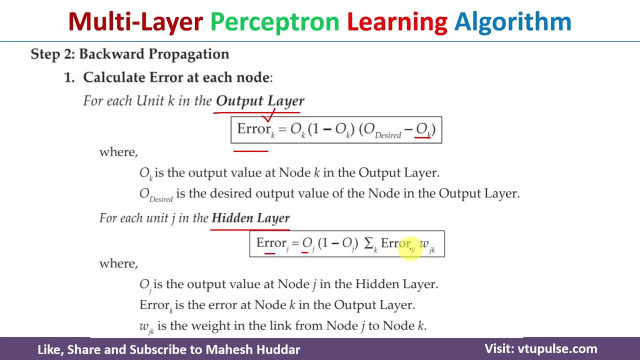 which is calculated in the output layer neuron. so error, the hidden layer neuron, error j is equivalent to oj multiplied by 1 minus oj. we have already calculated the output at each hidden layer neuron. output here multiplied by summation of error k, w, j, k, for all k, k is nothing, but what all output layer. 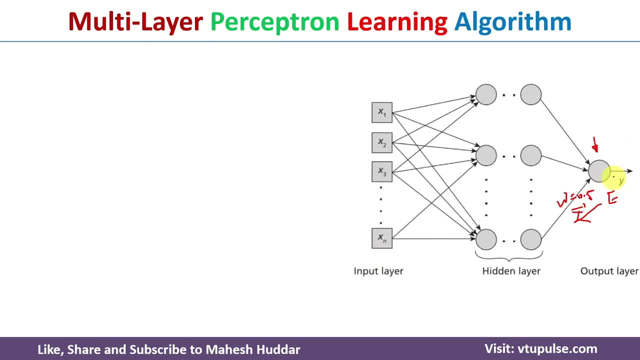 neurons here. so that is what i said. whatever the error we have calculated, the output layer neuron that will be propagated back with the proportion of the weight here. if the weight is equivalent to one, entire thing will be propagated back. if weight is equal to 0.5, 50 will be propagated back. 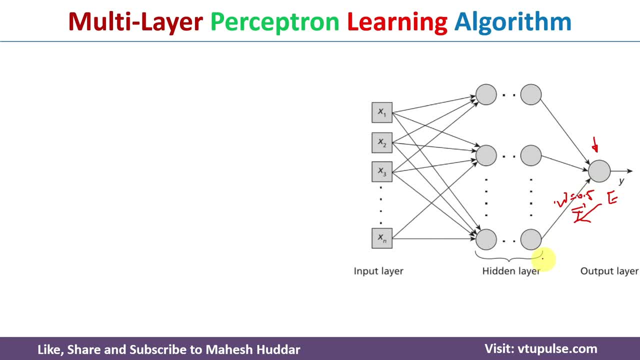 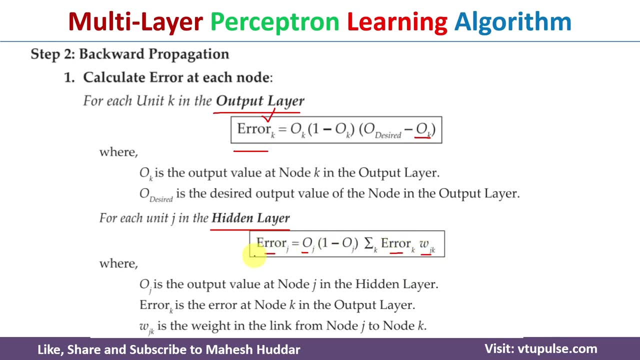 if it is 0.25, 25 percent will be propagated back, and so on. so that's the reason we have taken this error term. multiplied by the weight for all output layer neurons, we will get error at the hidden layer neuron in this case. once we calculate the error at the output layer neuron as well as the hidden layer neurons, the 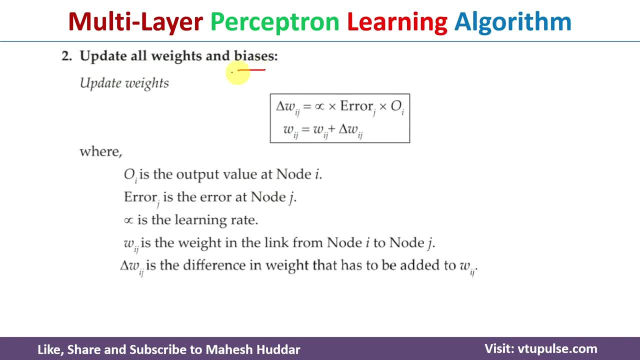 next step is to update all the weights as well as the biases here. so update the weights. we use this equation: delta w ij is equivalent to alpha, that is the learning rate multiplied by the error at that unit, that's the jth unit. multiplied by the input here you will get a change in weight. add that change in weight to the previous. 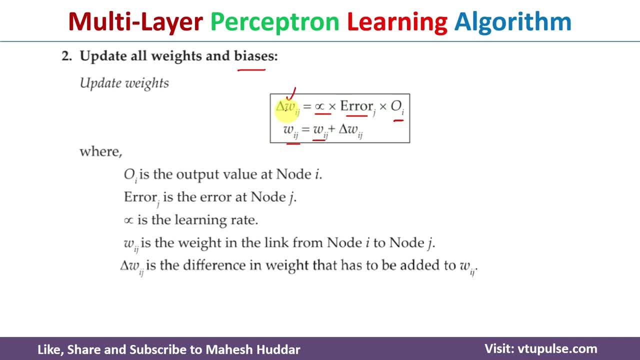 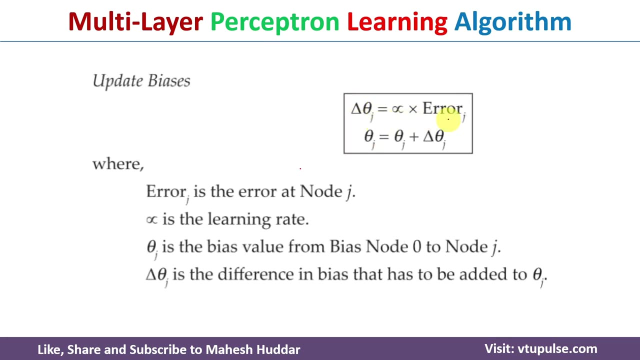 weight. you will get the new weight here, so this is the simplest process we follow to update the weights here. similarly, if you want to update the biases in biases, we don't have this input here. input will be always equivalent to one in that case. that is delta. theta j is equivalent to alpha multiplied.